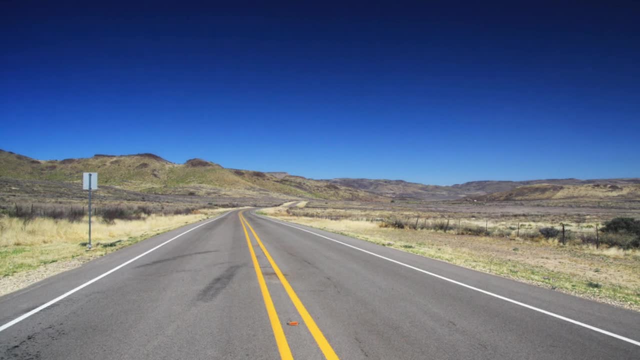 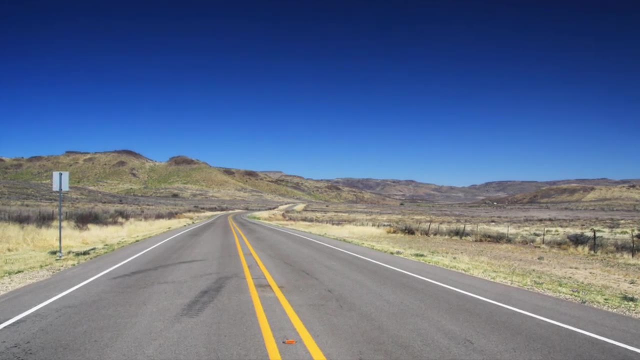 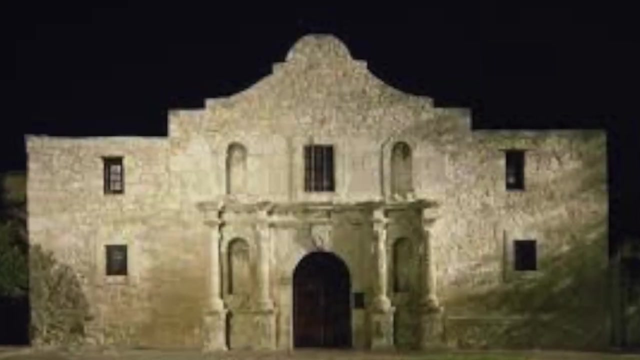 So in 1835, settlers living there rebelled. This was the beginning of the Texas Revolution. The settlers suffered a terrible defeat by the Mexican army at the 1836 battle at the Alamo, a mission in San Antonio, But the loss only inspired the settlers to continue to fight on. 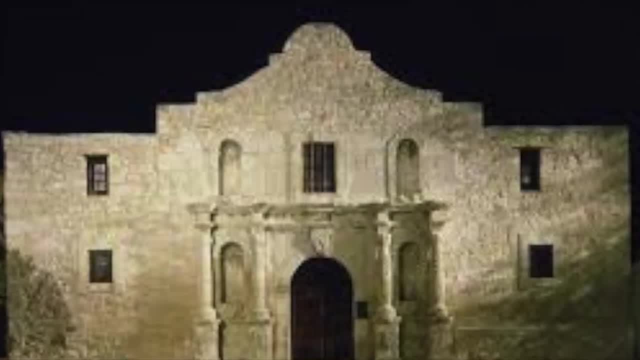 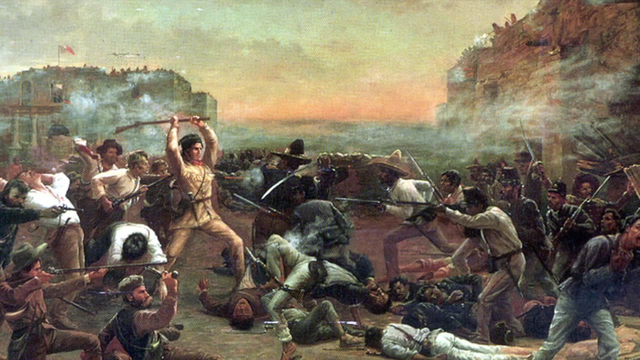 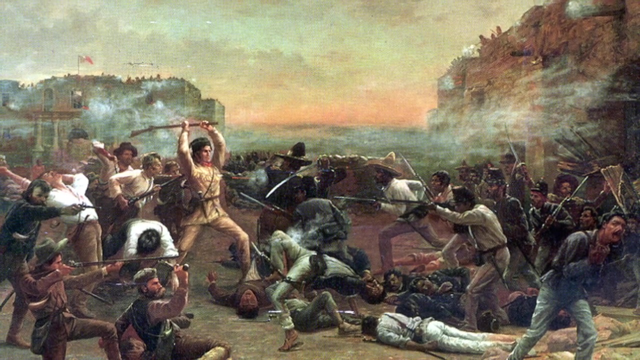 With a cry of Remember the Alamo. Many joined the rebel army, and soon Mexico gave up. On March 2, 1836, Texas declared independence from Mexico, and soon they were at war. Texas won, But Mexico refused to recognize Texas as an independent colony. 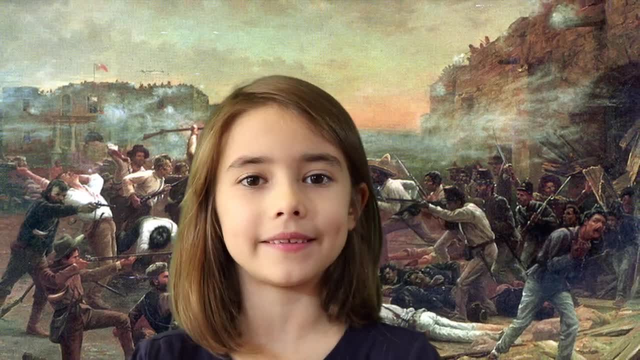 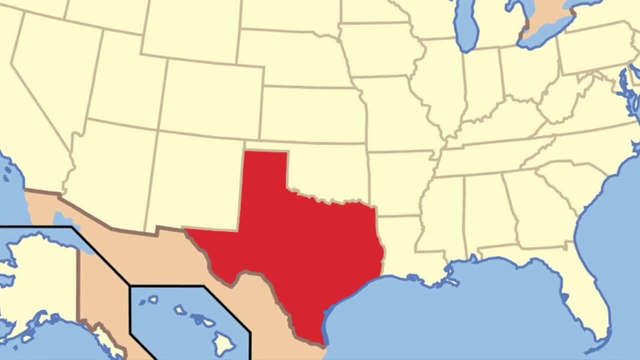 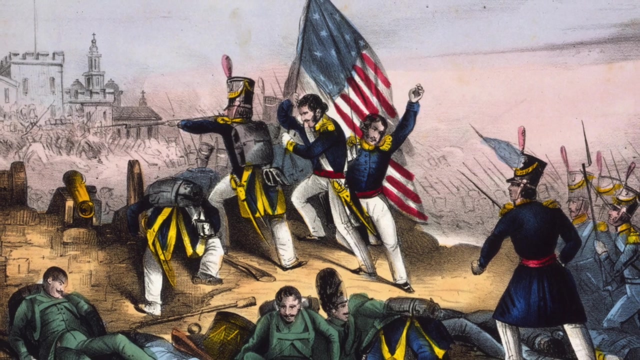 Texas then asked to become a state of the United States. It was years later. in 1845, the US added Texas as a state and Mexico broke off their diplomatic relations. Mexico didn't want to take any offers from the US to buy land extending from Texas to the Pacific Ocean. 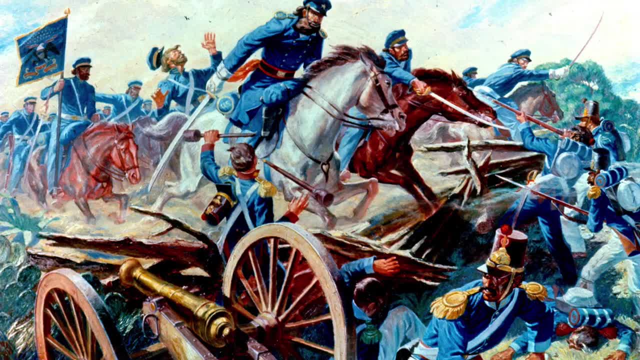 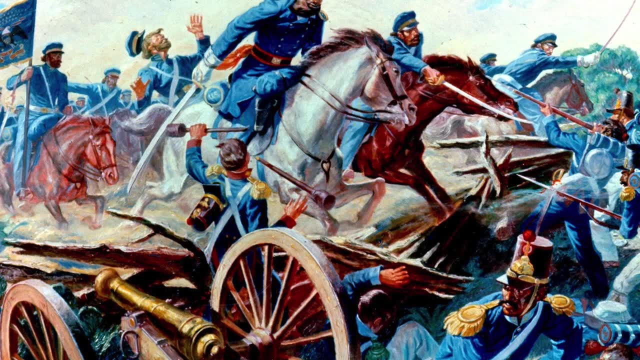 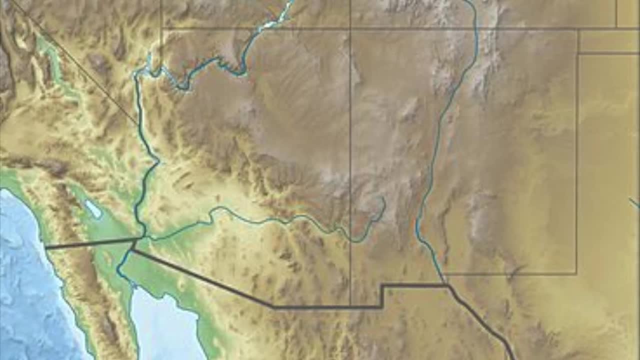 In 1846, a fight over the border between Texas and Mexico resulted in an armed conflict and the Mexican-American War. The United States won this war and, by the Treaty of Guadalupe, Hidalgo won lands that later formed the states of California, Arizona, Nevada, Utah, New Mexico. 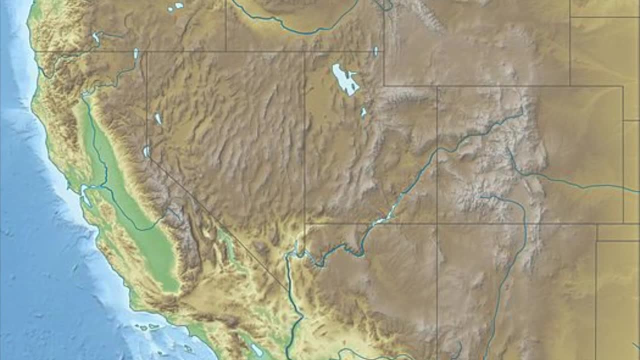 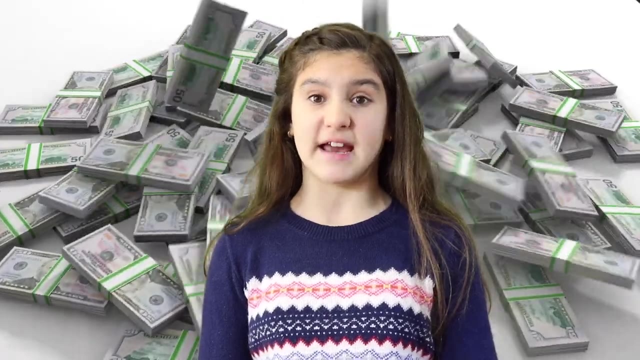 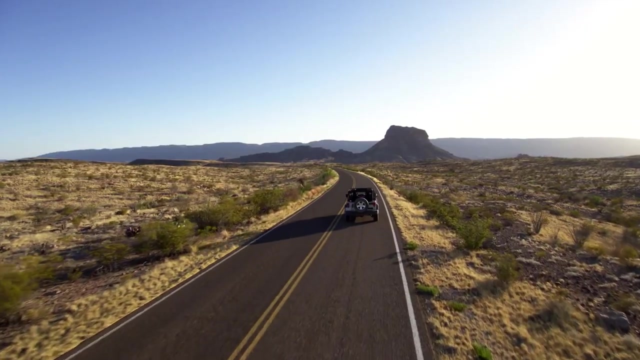 as well as parts of southwestern Colorado and southwestern Wyoming. Mexico was given $15 million to give up its claims to Texas. $15 million, That's a lot of money. Obtaining Texas independence was a long process, beginning in 1824 and ending in 1848. 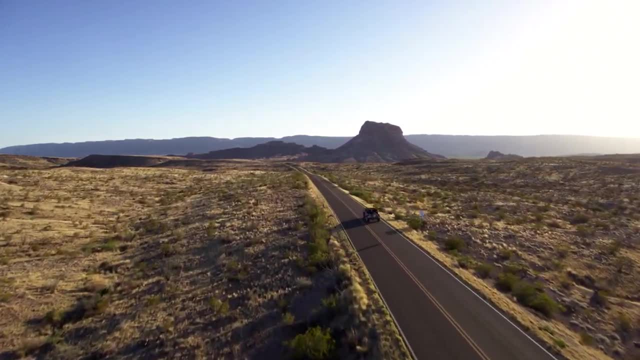 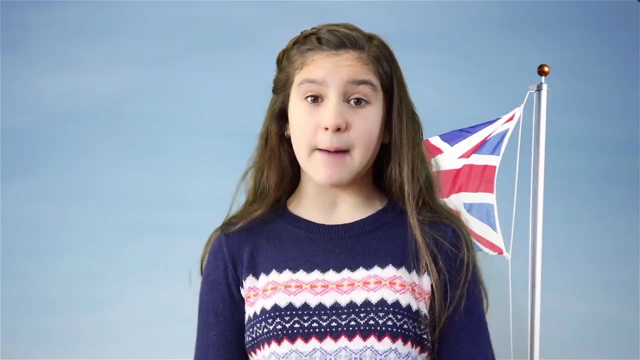 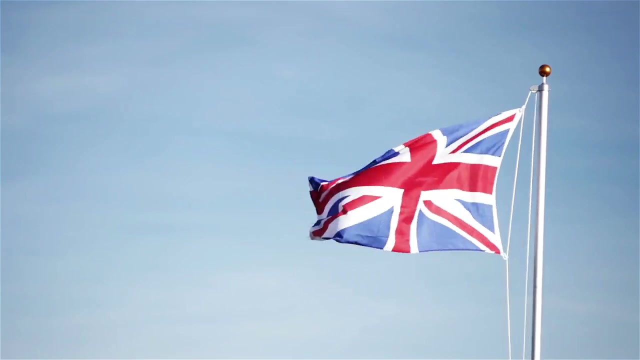 Leaders like Sam Houston and Stephen F Austin gained the support of other Texans who shared their same beliefs. They had settled in Texas to establish new lives from the persecution of England. They banded together because they wouldn't tolerate the removal of their new freedoms by Santa Ana. 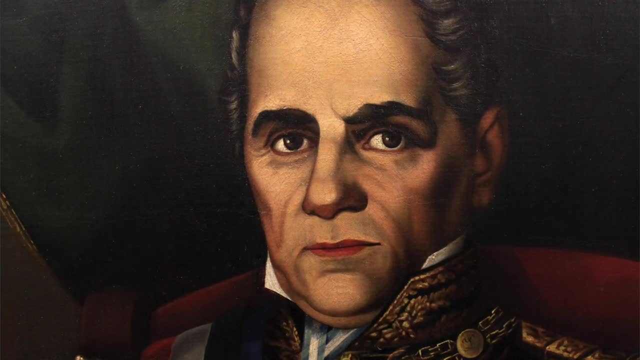 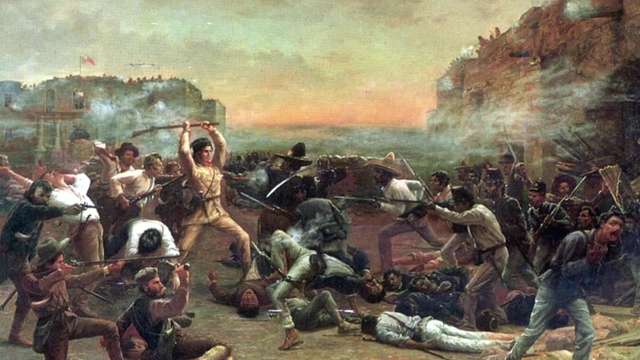 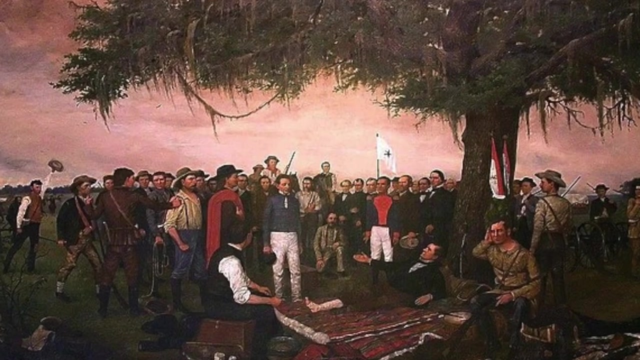 the Mexican president of Texas, Santa Ana, was trying to gain more powers over the people in Texas. This was exactly what they had already been trying to escape from England. After many battles in places like the Alamo, the Texans were able to gain their independence from Mexico. 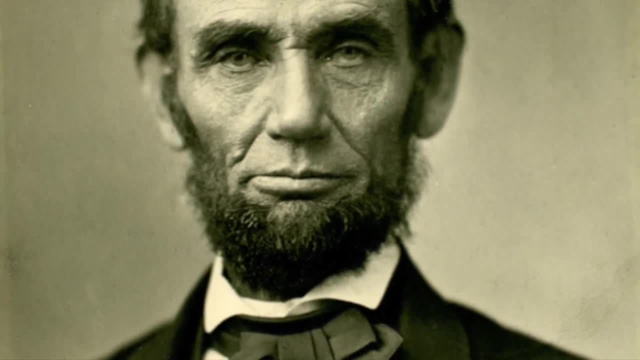 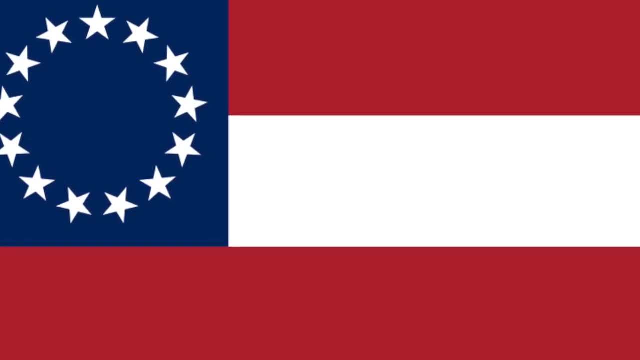 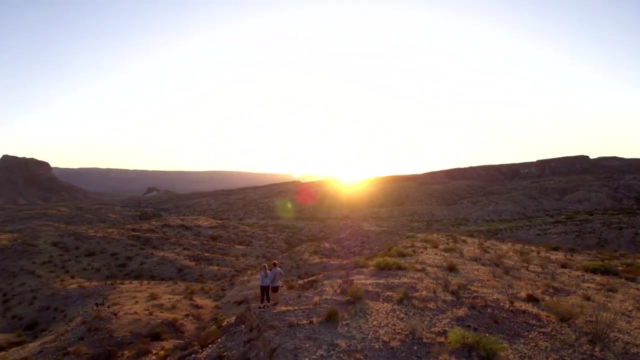 And after Abraham Lincoln was elected President of the United States, Texas joined the newly formed Confederate States of America in 1861 and fought in the American Civil War, trying to become independent from the United States. The Confederates lost to the Union in 1865,. 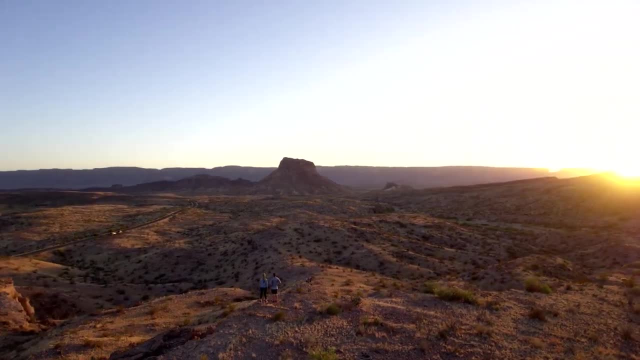 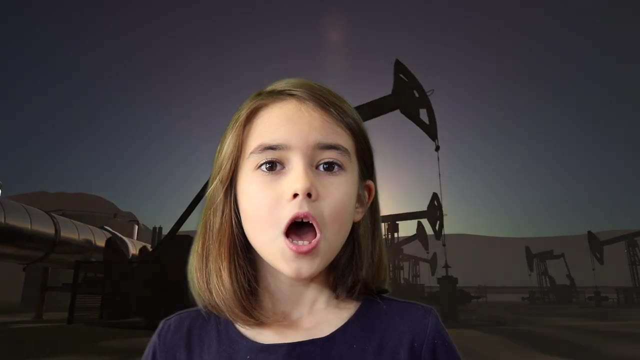 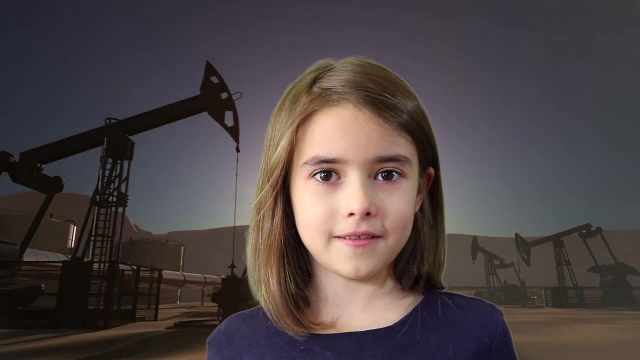 and Texas was restored to full representation in Congress on March 30, 1870.. On January 10, 1901, oil was struck in Texas. This led to the founding of a richer economy During a time when the economy was bad. many people left Texas left Texas For many years. Texas lost much of its population. It wasn't until the 1950s and 60s that people started to repopulate Texas and move back. Recently, Texas has been exploring technology and computers. The land that is now Texas has been inhabited for many, many years. People first came to what is now Texas at least 16,700 years ago. Thousands of years later, Native American tribes including the Okokisa, Karankawa, Mogollon and Comanche lived there. 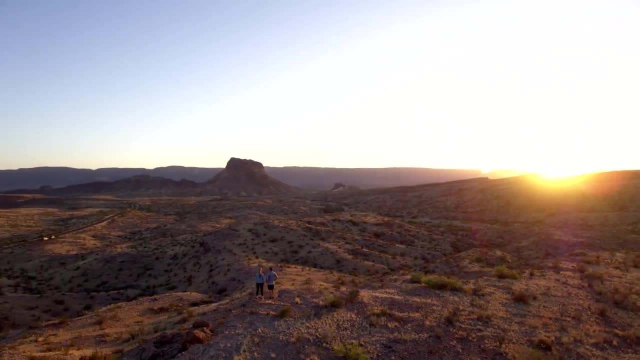 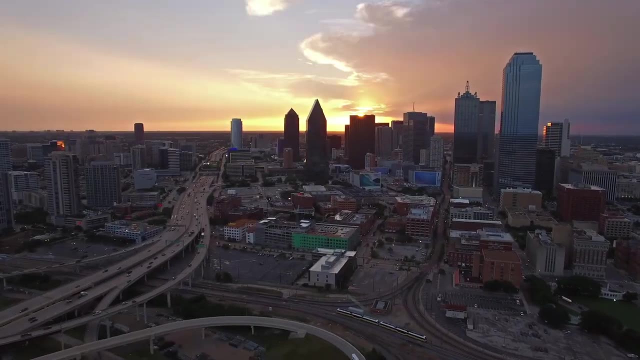 Spanish settlers promoting Christianity, called missionaries, were some of the first Europeans to live in what is now Texas. So how did Texas get its name? Well, around 1540, in the area that is now East Texas, Spanish explorers met the Caddo Indians. The Caddos called the Spanish Teixas, meaning friends or allies. In Spanish, this actually translated to Tejas, And the United States eventually converted this name to Texas Tejas. Like Jose Tejas, I love Jose Tejas. 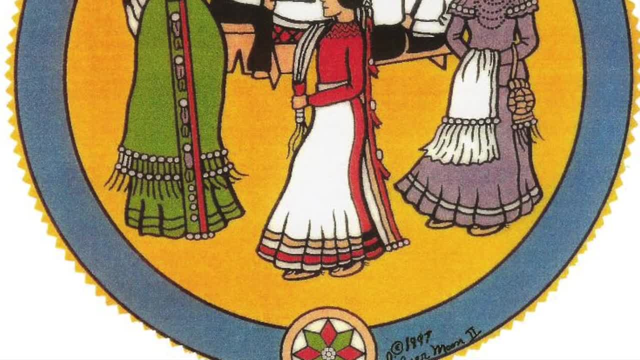 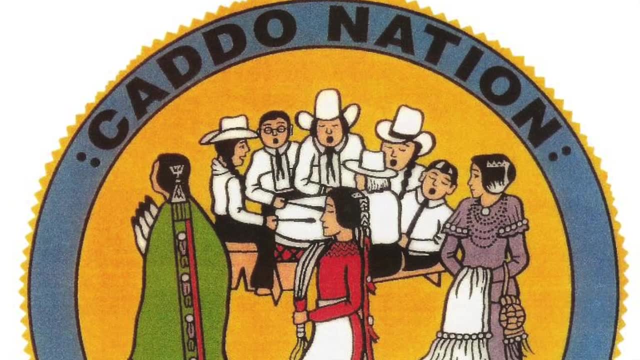 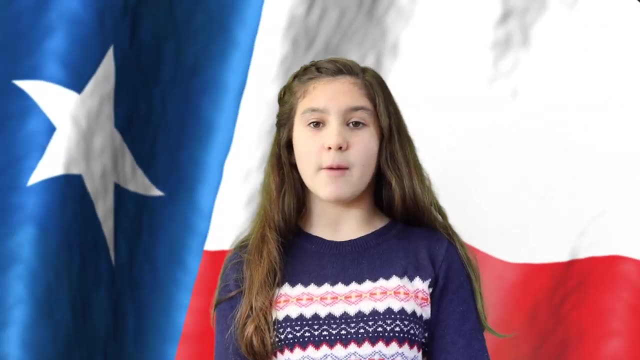 Many believe that the Caddo tribe greeted Spanish settlers by saying Tejas, which means friends, and kind of sounds like Texas. Texas is called the Lone Star State because in 1836, when the Republic of Texas declared itself an independent nation, it flew a flag with a single star in it. 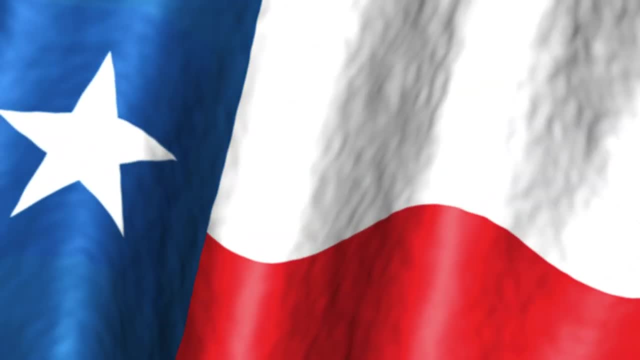 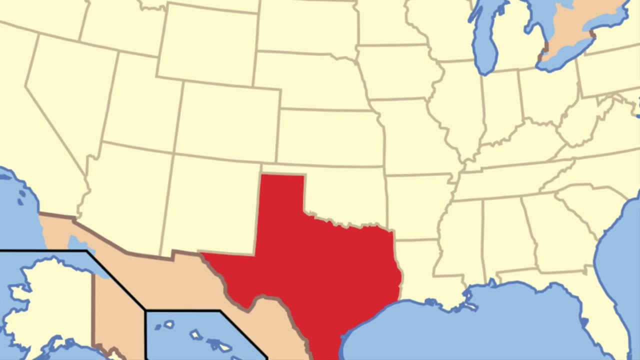 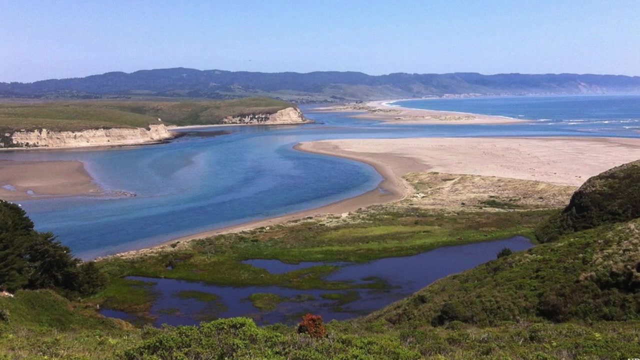 The Lone Star can be found on the Texan state flag and on the Texan state seal. New Mexico borders Texas in the northwest, Oklahoma in the north and northeast, Arkansas, Louisiana and the Gulf of Mexico in the east and Mexico in the southwest. 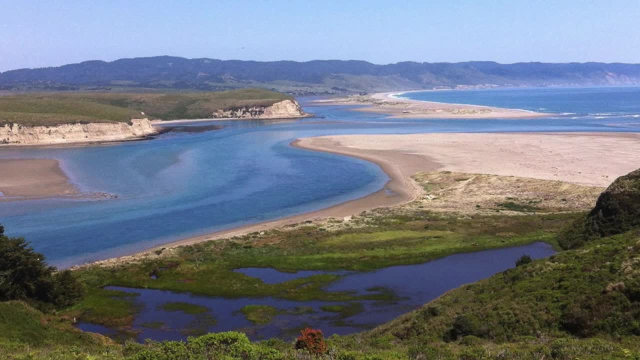 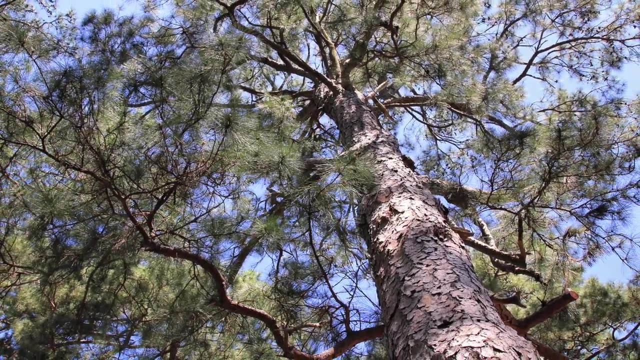 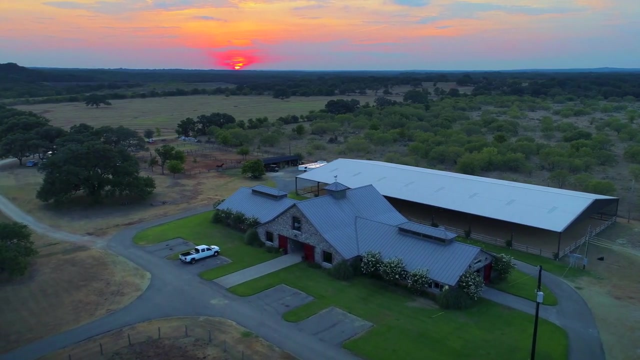 The hilly southern and eastern part of the state is called the Gulf Coastal Plains. This includes the Pine Belt where most of Texas' commercial timber grows. The interior lowlands cover the northeast and have some of the state's largest ranches. The Great Plains stretch across the north and west parts of the state. 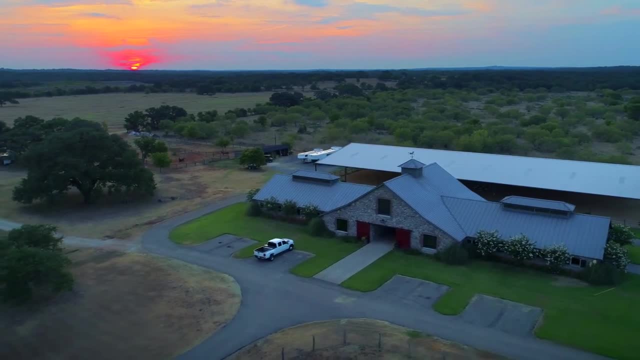 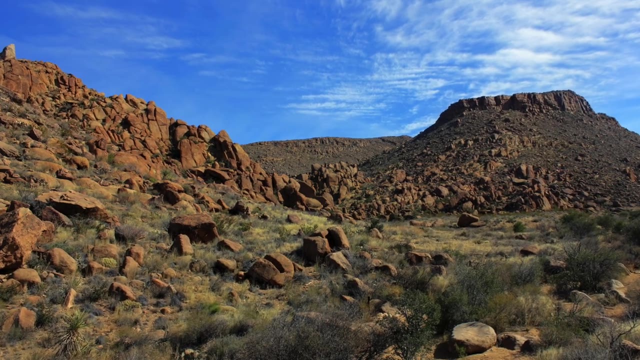 but these extend all the way to Canada. Far west is the Basin and Range Province. This is Texas' only mountainous region. It's bordered on the south by the Rio Grande, the river that marks the boundary between the United States and Mexico. Texas is the only state to have the flags of six different nations to fly over it: Spain, France, Mexico, the Republic of Texas, the Confederate States and the United States. When Texas joined the Union, it kept the right to fly its state flag at the same height as the national flag. 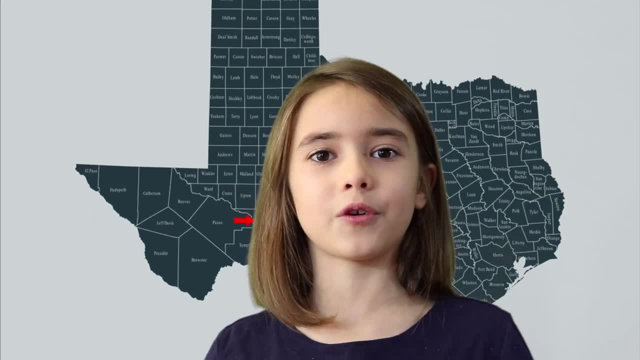 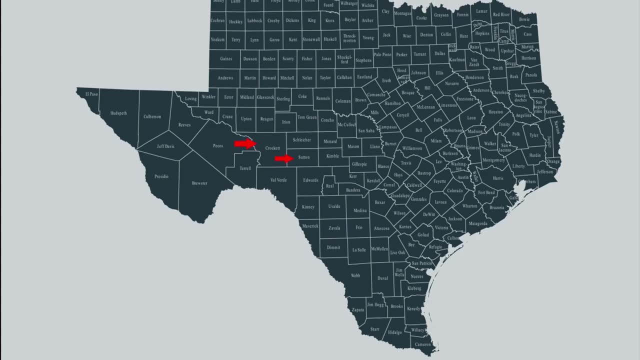 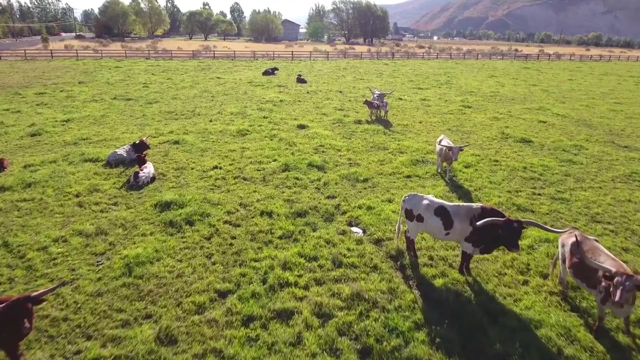 Did you know that Texas has 254 counties? This is more counties than any other state in the US? Texas leads the nation in the production of cattle. Due to its long history as a center of the cattle industry, many people associate Texas with the image of cowboys. About 27 million people live in Texas. It's larger than France. In 1845, it became the 28th state in the United States. The largest cities in Texas are Houston, Dallas, Fort Worth, San Antonio, El Paso and Austin. 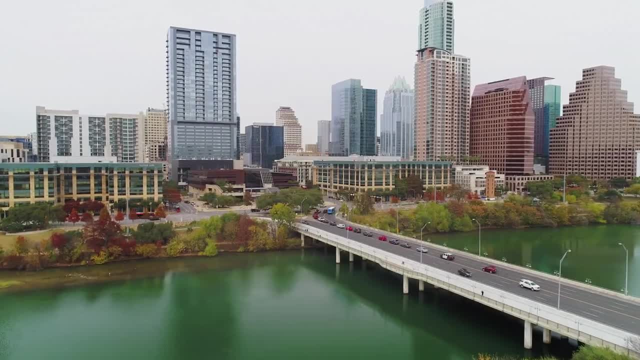 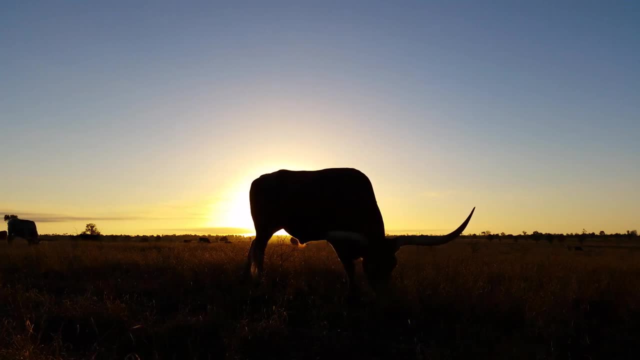 Austin is the capital city of Texas. There are many famous attractions in Texas. Fort Worth is known for its stockyards and Amarillo is known for the cattle business and stockyards. In Dallas, industrial technology companies such as Texas Instruments and EDS have their offices. 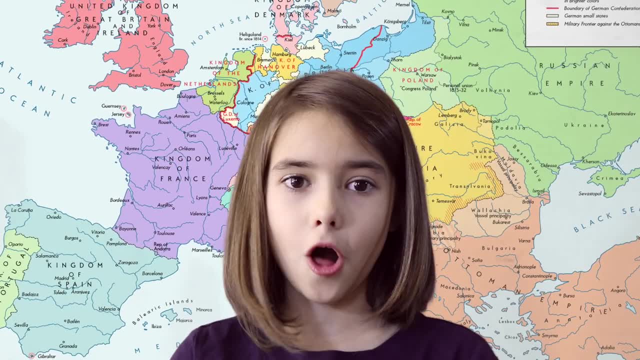 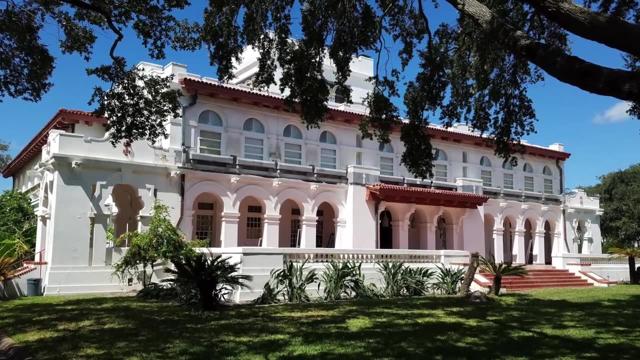 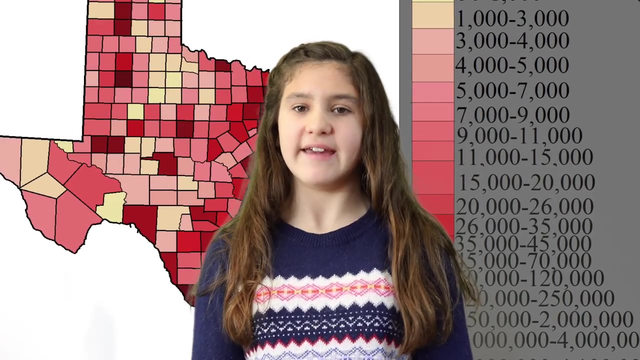 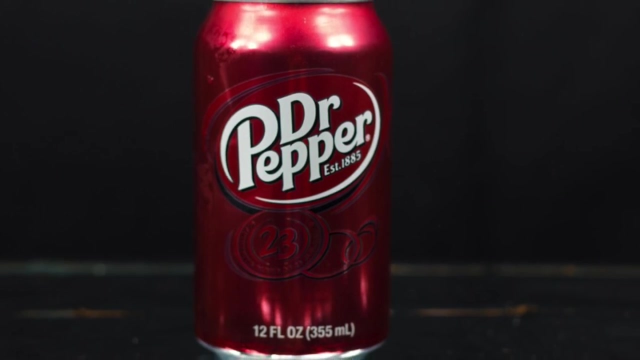 Hey, guess what? Texas is bigger than any other country in Europe. King Ranch in Texas is bigger than the entire state of Rhode Island. Texas also has the second largest population in the USA. California has the most. The soda Dr Pepper was invented in Waco, Texas, in 1885 by a pharmacist named Charles Alderton. 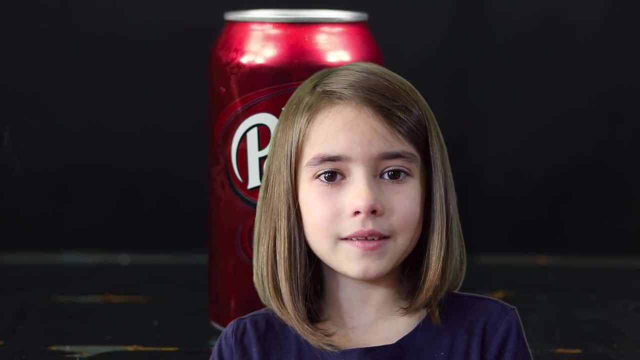 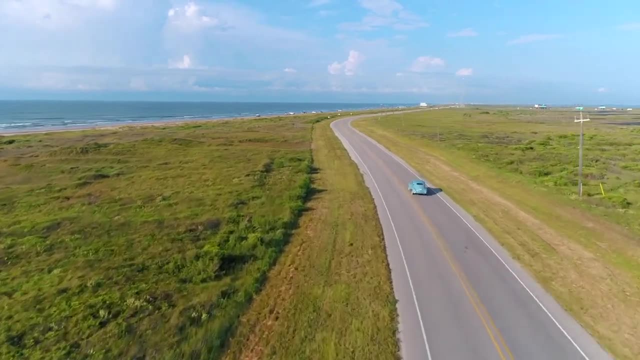 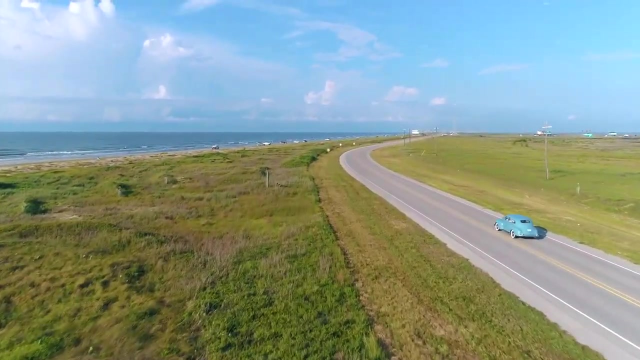 A very popular snack in Texas is peanuts inside the Dr Pepper. Did you know that Texas has more than 70,000 miles of highway And each year the state uses 1.6 million dollars of white and yellow paint to line its highways? 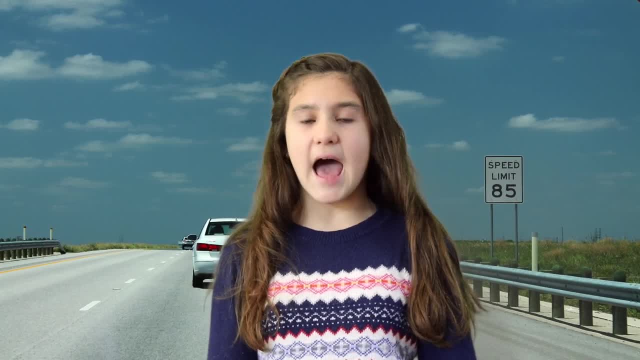 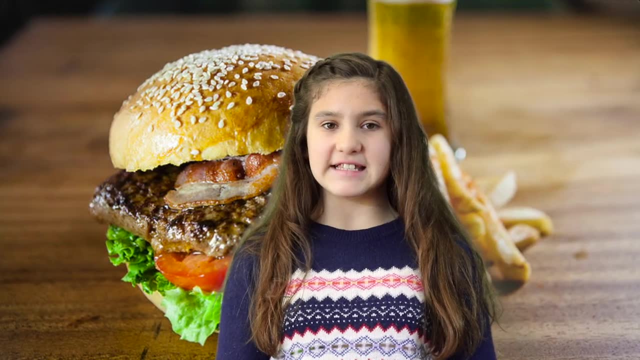 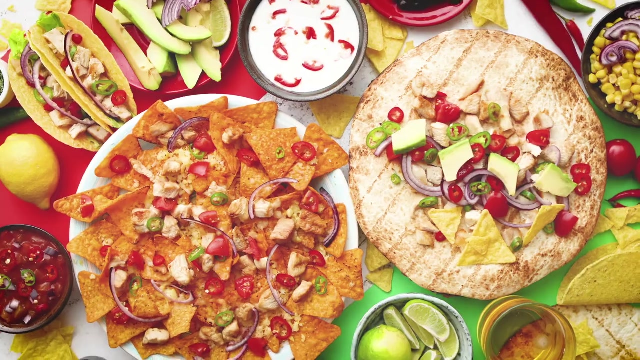 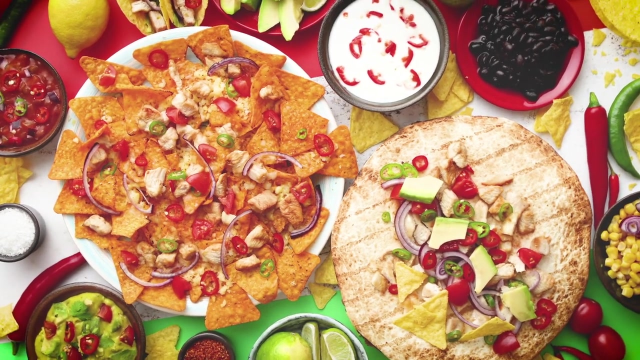 Hey, guess what? Texas also has the highest speed limit in the country: 85 miles per hour. Athens. Texas claims to be the birthplace of the hamburger. I love hamburgers. Texas is also known for Tex-Mex food, a combination of Texan and Mexican cuisine that includes nachos, fajitas.